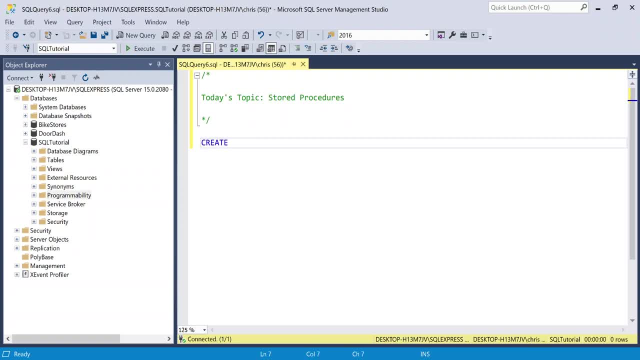 complicated. So the very first thing that you need to write is create, and then procedure, And after that you're going to name it. Let's just call this one test- And all you're going to say is as: and then you're going to write your query, And so let's just do select as. 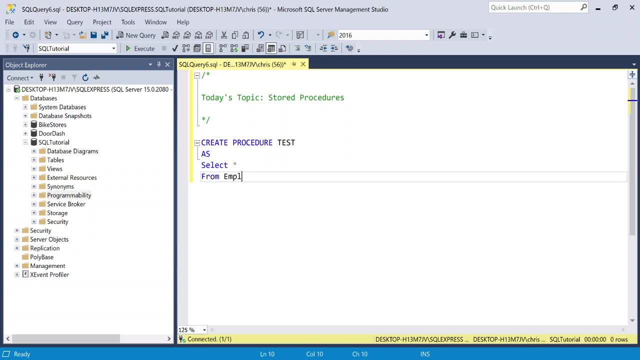 Everything from employee demographics, And that is it. We have created our very first stored procedure. Of course, this is super, super simple, But let's execute this really quick and take a look at it, So it says that the commands completed successfully. Let's go over to our SQL tutorial. 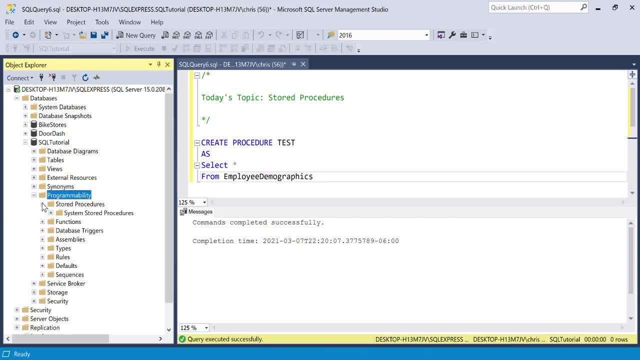 We're going to go over to programmability, stored procedures, and it is not showing up there. What we need to do is we need to refresh our stored procedures. We're just going to go right here, I'm going to click refresh And then there is our stored procedure. Now, how do you actually use? 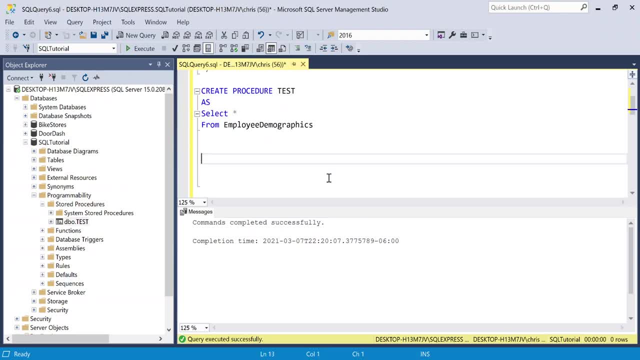 the stored procedure that we just created. So let's go right down here And let's say X, which means execute, And then all we're going to say is test, And we're going to run this, And there we go. So all we put in this stored procedure was a select statement, And so when 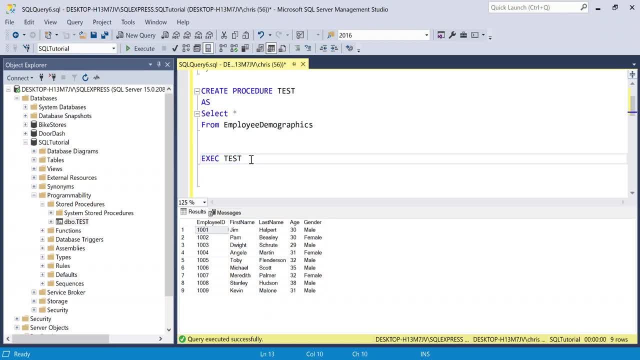 we actually ran the stored procedure. it returned our select statement. Now let's go down here. We're going to make it a little bit more complicated. We're going to do the exact same thing in create stored procedure- Make sure I spell that right. And let's call this temp underscore employee. So if you remember from 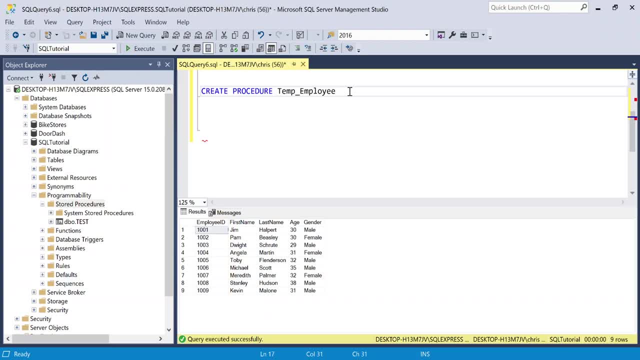 a previous video we worked on temp tables and we created our temp tables, then inserted data into that. we are going to add that to this stored procedure So we can see the difference between a simple query versus a little bit more complicated query. So I'm going to say as, and then I'm going 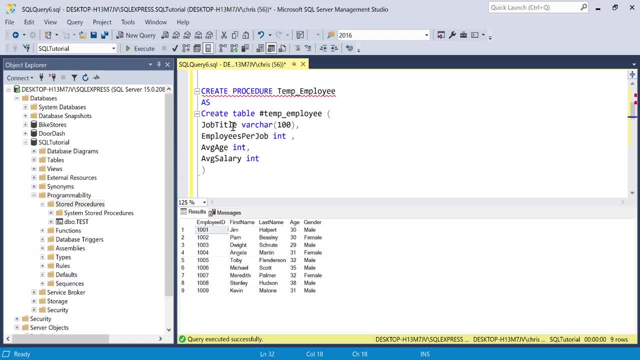 to insert that in here. Now, what this is doing is I'm creating a table And then, right down here, I'm inserting that table. Now, if I create this stored procedure and then execute it, nothing is actually going to be returned. it will insert the data into that temp table, But since I don't have a select statement, 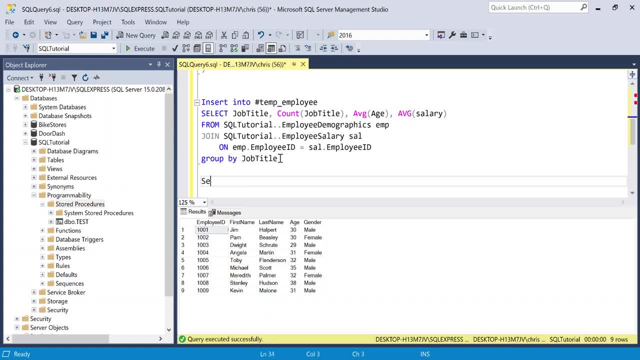 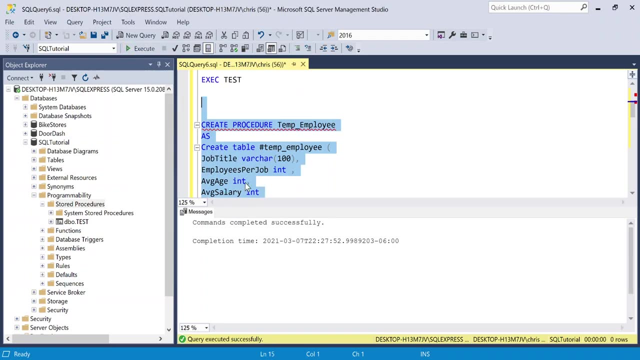 in this stored procedure, nothing will be returned. So let's write: select everything and we'll just do from and this is temp employee, And right here And so now let's create our store procedure So that created successfully, Let's refresh over here And let's execute this. So let's. 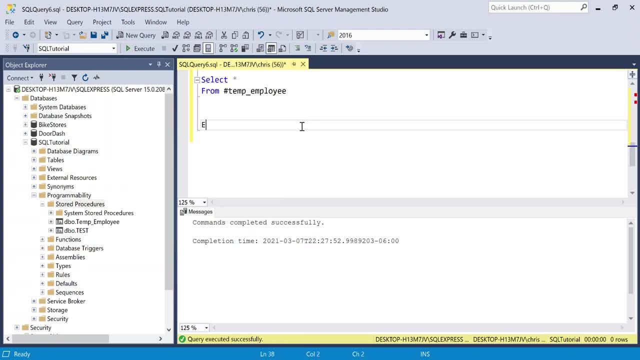 just go down right here And say execute, and it's going to be temp employee, And now we will execute this And there is our output. Now, really quick, let's go into temp employee And we actually want to change this stored procedure. So we're going to go over to modify. So when we modify, 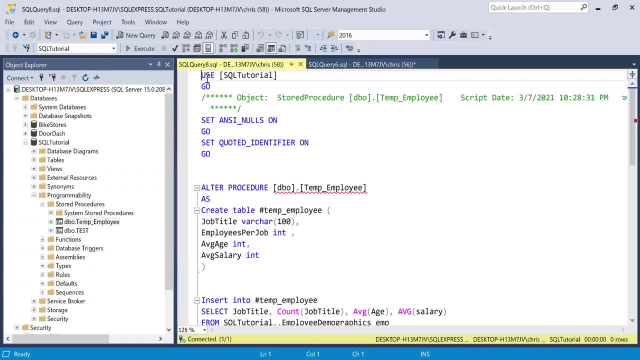 it. a few things are going to show up on your screen. The first thing that you're going to see is it says use SQL tutorial. So it's just specifying the database. The next two things you may not be as familiar with. it's set ANSI nulls and then set quoted identifier. If you don't know, 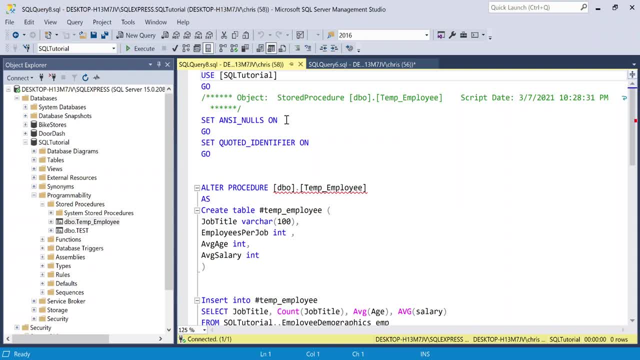 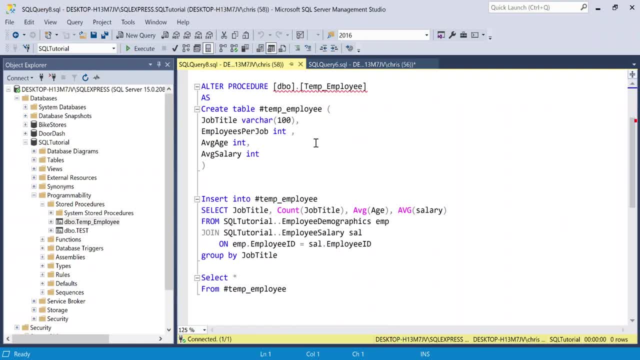 we're going to look at the alter procedure. So we created our store procedure but now we want to alter it. So this is the alter procedure And we're going to add a parameter to this. So what the parameter is going to allow us to do is when we're actually executing the store procedure. 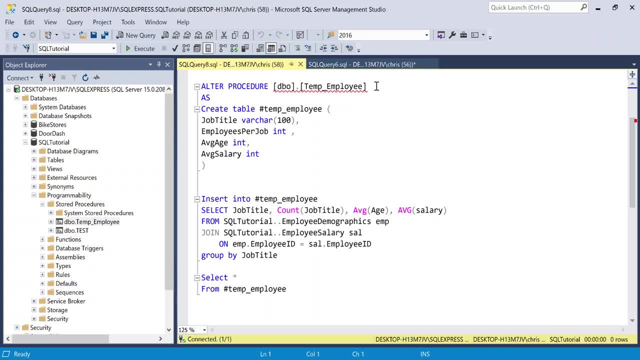 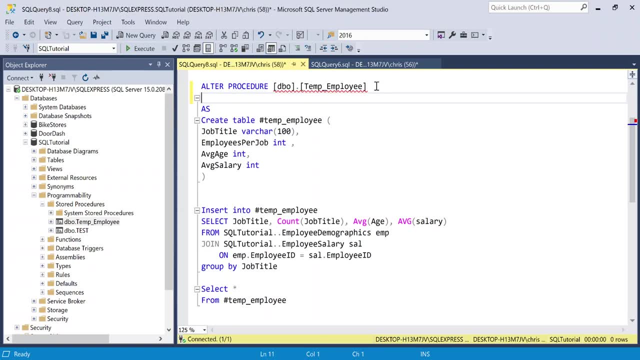 we can specify an input into that store procedure so that we get a specific result back, And I'm going to show you what I mean by that in just a second. But let's actually add our input And let's just say job title, And we need to specify the data type that that is going to be. So let's. 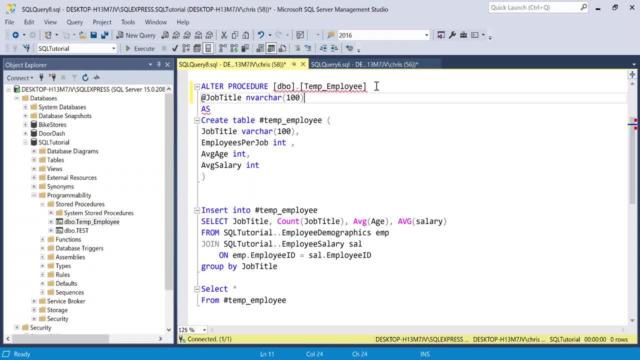 just say nvarchar 100.. I know below it says varchar 100, but that's not extremely important. So this is going to be our input. So we need to go down here and say where job title is equal to at job title. So when we actually are executing this and we say the job title is equal to, let's say, a count.